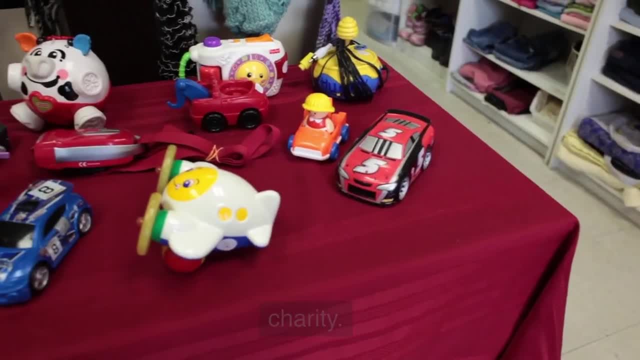 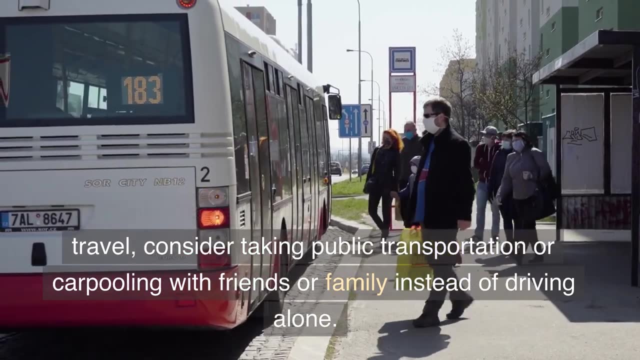 make extra money or donate them to a thrift store or charity. Use public transportation or carpool If you have to travel. consider taking public transportation or carpooling with friends or family instead of driving alone. This can save you money on gas and. 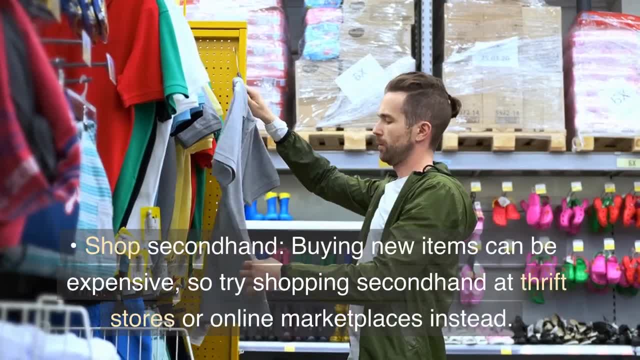 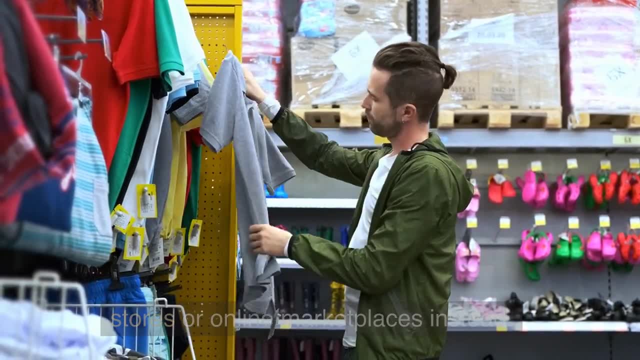 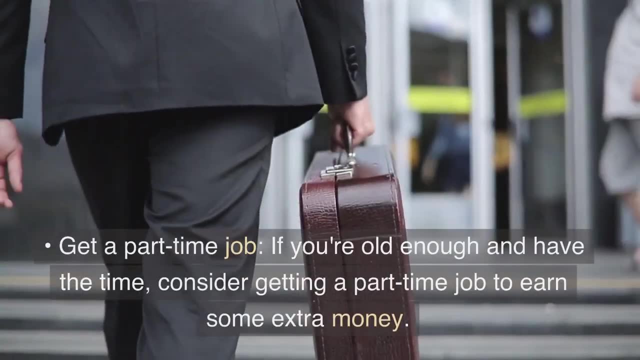 wear and tear on your car. Shop second-hand. Buying new items can be expensive, so try shopping second-hand at thrift stores or online marketplaces instead. You can often find gently used items for a fraction of the cost of new ones. Get a part-time job If you're old enough and have the time. consider getting a part-time job to earn some extra money. 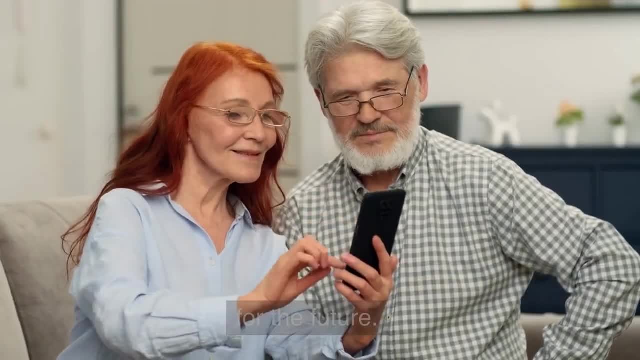 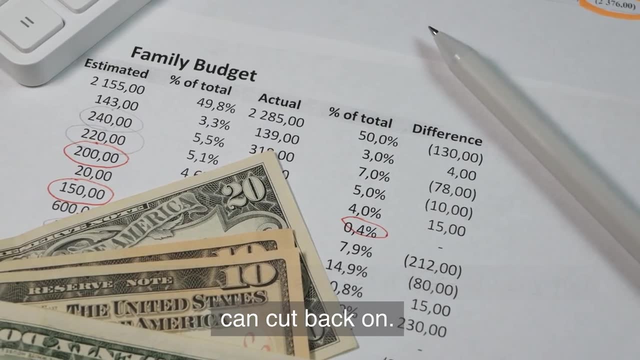 This can help you save up for a big purchase or save for the future. Cut back on unnecessary expenses. Take a look at your monthly expenses and see if there are any you can cut back on. Maybe you're paying for a subscription you don't use or you're buying more groceries than you need. 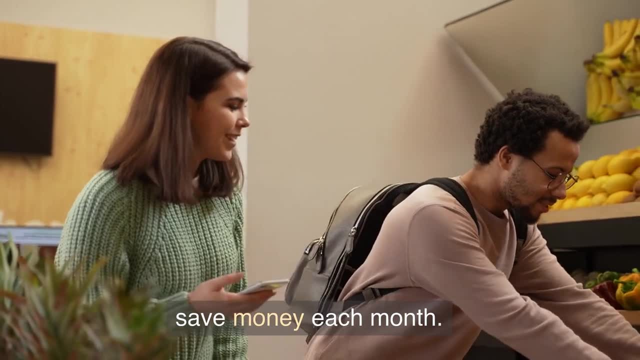 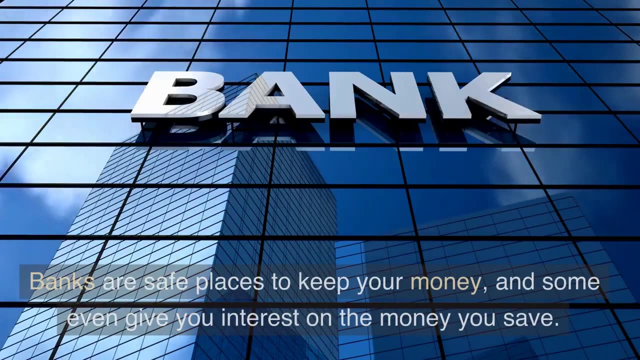 Cutting back on unnecessary expenses can help you save money each month. When you have a lot of money saved up, it might be a good idea to put it in a bank. Banks are safe places to keep your money and some even give you interest on the money you save. 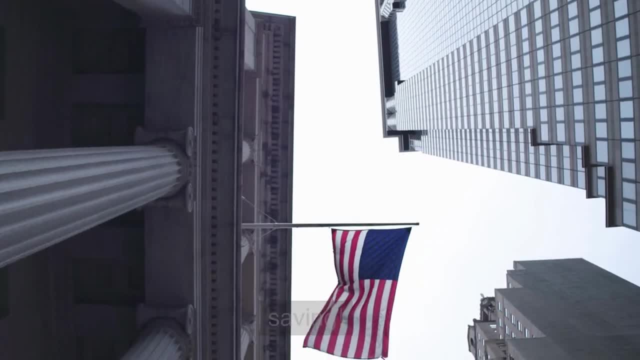 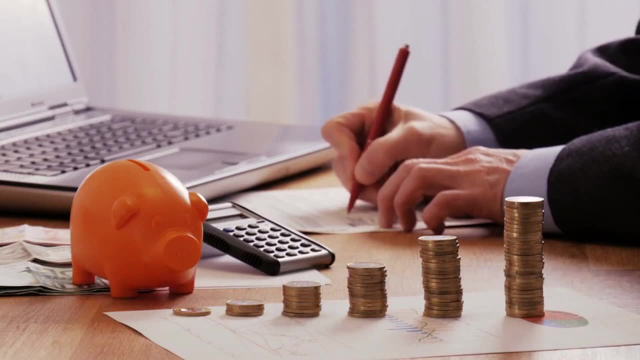 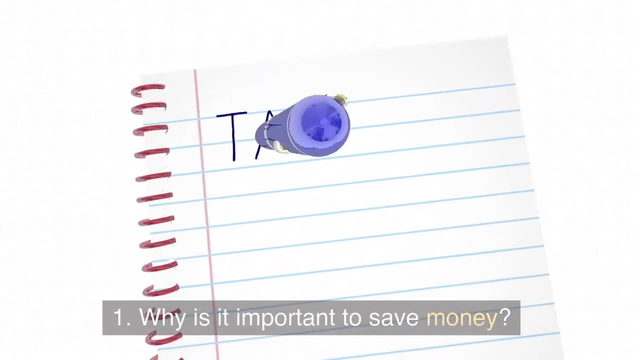 This means you can earn even more money just by saving. Remember, saving money is all about being smart with your spending and making your money work for you. Now it's time for a quiz. See how much you learned about saving money. 1. Why is it important to save? 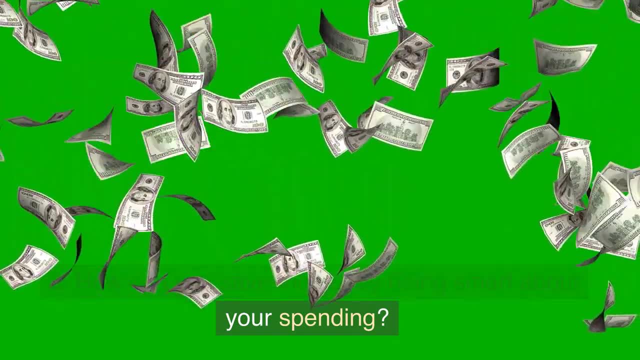 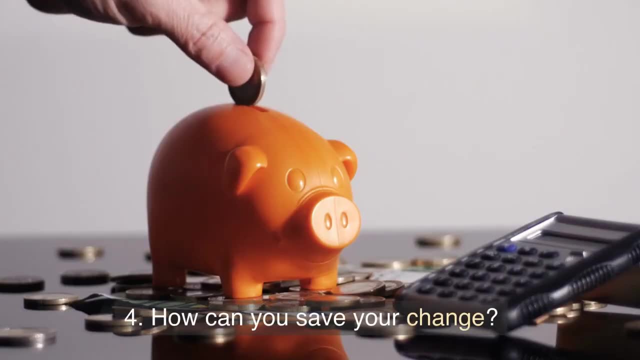 2. How can you save money by being smart about your spending? 3. What is a budget and how can it help you save? 4. How can you save your change? 5. What are some ways you can save your money in a bank? 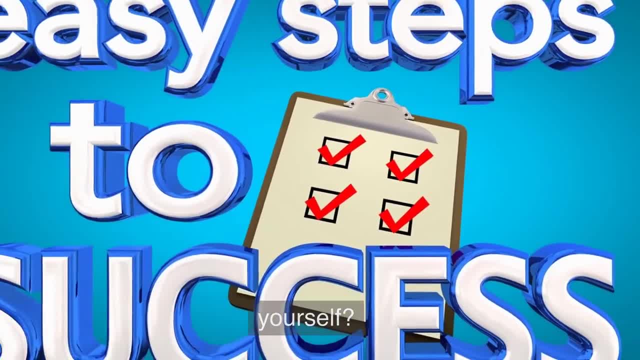 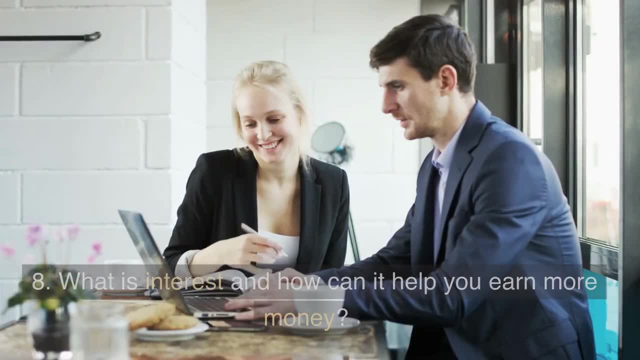 6. What are some tips for setting saving goals for yourself? 7. How can you save money on your allowance or money you get from doing chores? 8. What is in your bank? 9. What is your interest and how can it help you earn more money? 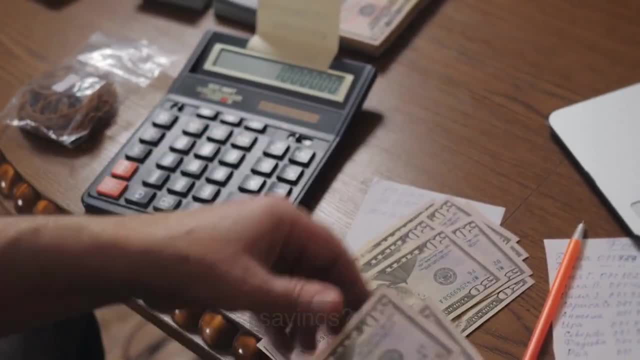 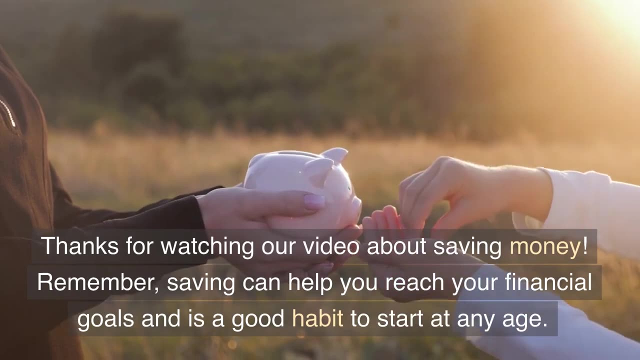 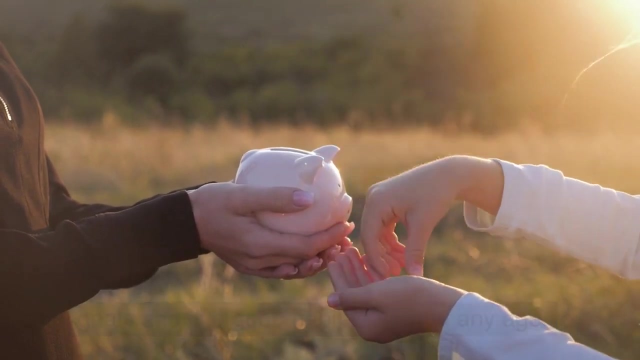 10. Why is it a good idea to set a specific goal for your savings? 9. What are some ways you can save money for the future? Thanks for watching our video about saving money. Remember, saving can help you reach your financial goals and is a good habit to start at any age. Like the video and subscribe to our channel. 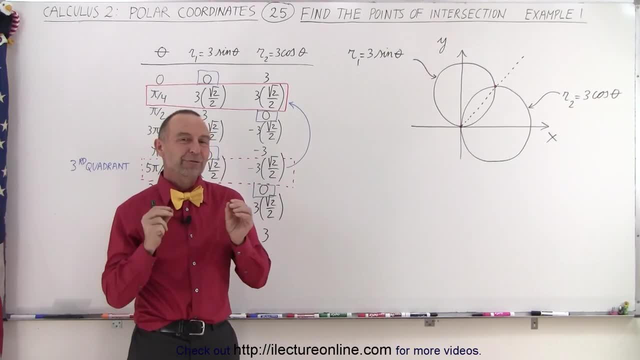 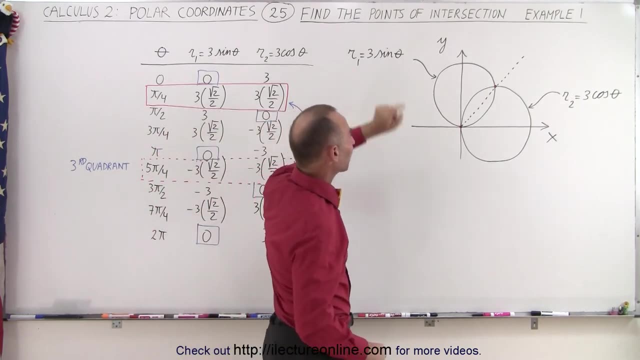 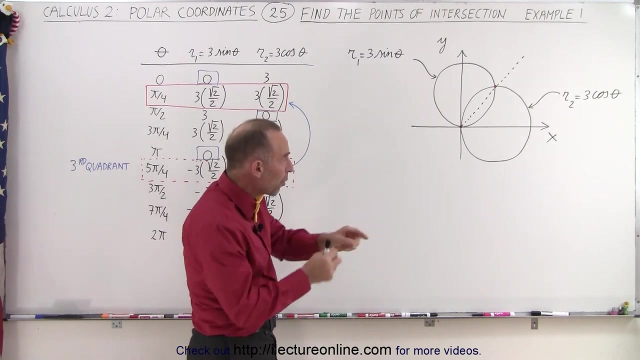 Welcome to Electron Line. Here we're going to find the points of intersection of two polar equations. The two equations are R1, three times the sine of theta and R2, three times the cosine of theta. They're both circles, They both have a point on the origin and then you can see that the cosine function is along the x-axis. 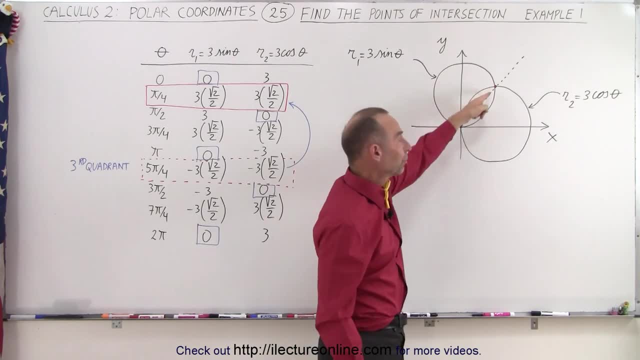 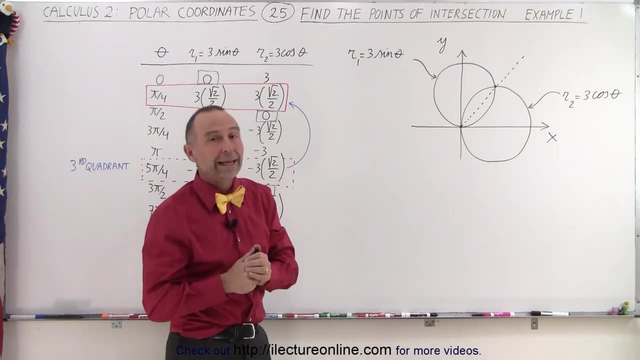 the sine function is along the y-axis and they do intersect at two different places. Now let's say you did not draw the two graphs and you really didn't know what they looked like and you wanted to find the points of intersection. It turns out when we try to find the points of intersection for polar equations or polar graphs, 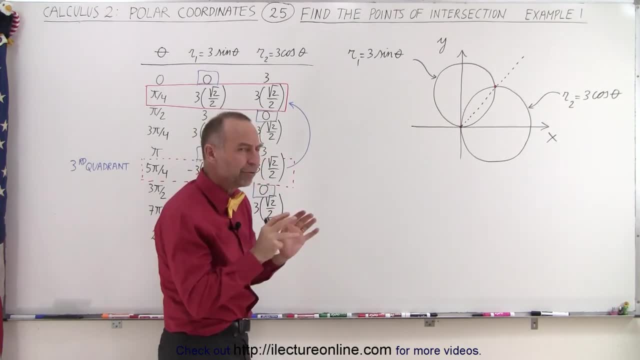 it's not as easy as you think. it might be A little bit of confusion there, so I'm going to try and explain why there's this confusion and how to deal with it. Well, first of all, let's go ahead and do it the way we'd normally do it for any sort of coordinate system. 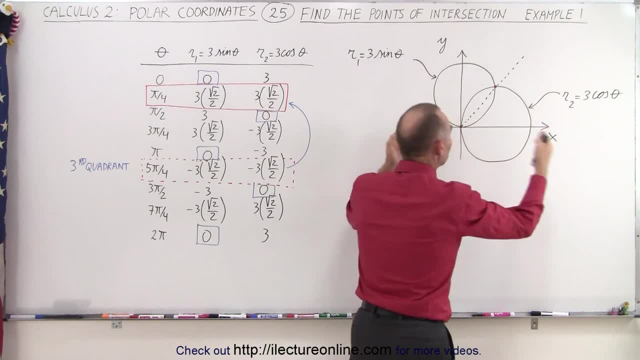 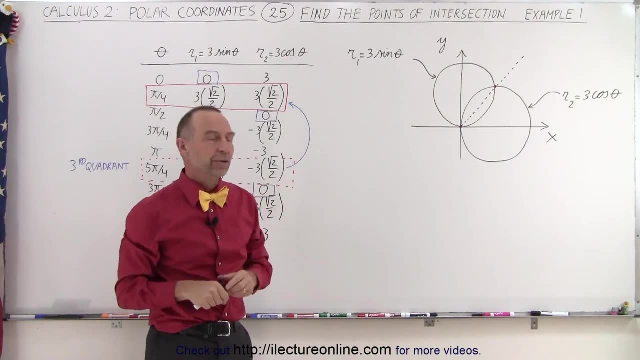 We simply set the two equations. They're equal to each other to see for what value of the independent variable, in this case theta- they have a common point on the graph. So we're going to set R1 equal to R2 and then solve that simultaneously.